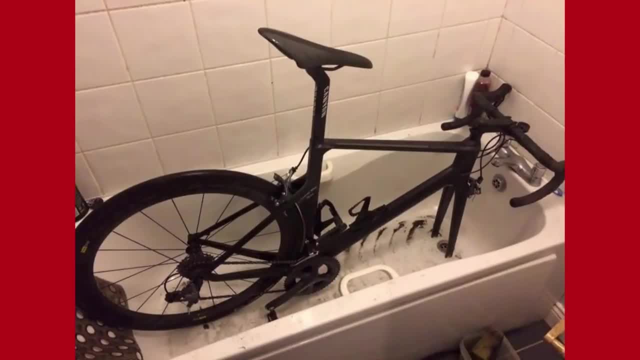 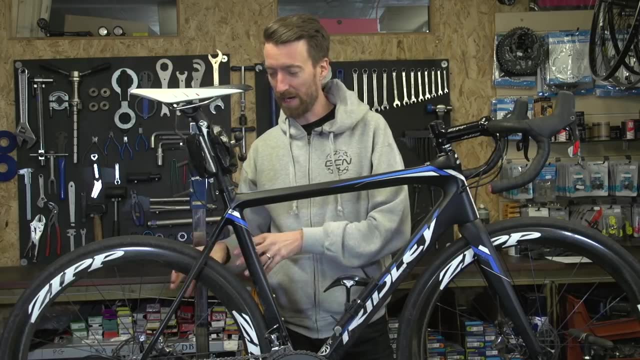 However, we would recommend checking with your partner or family before you do this, before you get yourself into lots of trouble. Now, along with lubricating your chain and some of the other moving parts in the drive tray, there are other parts on the bike which will need grease or some kind of grease. 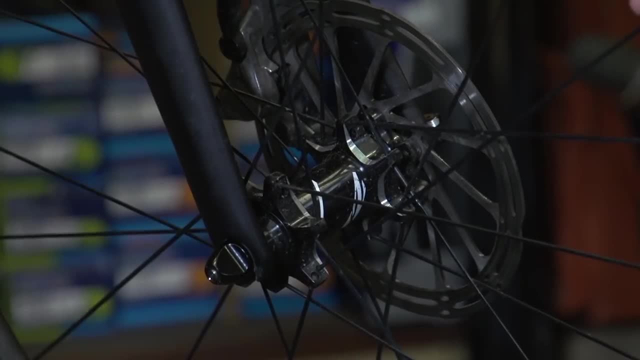 which will need grease or some kind of grease which will need grease or some kind of grease like grip paste. So I'm thinking things like the hubs, the headset bearings here, or the grip paste that you can put down on a carbon seat post. 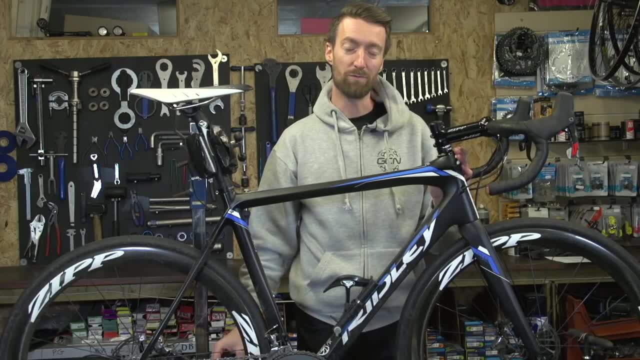 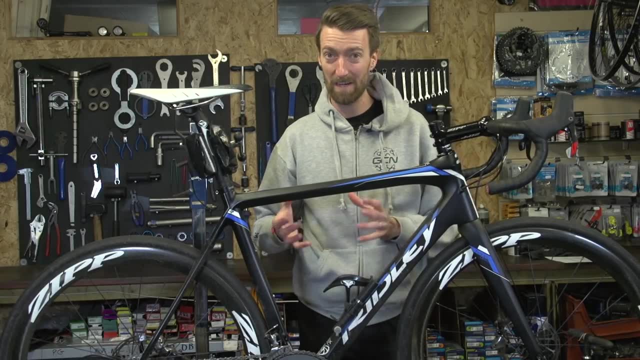 to stop it seizing, and also in the threads of things like pedals as well. Now you can prolong the grease lifespan by avoiding jet spraying directly towards these parts, But even if you do avoid doing that, it's still not a bad idea every so often. 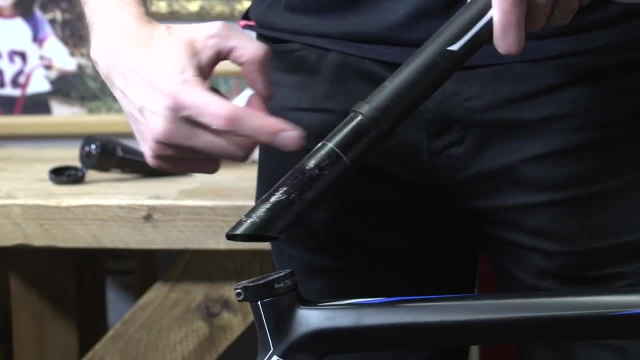 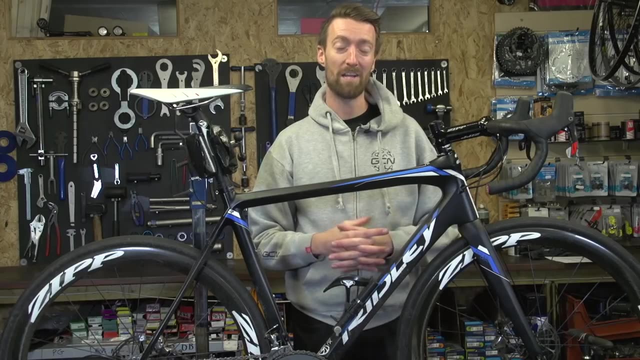 to take them apart, clean them and reapply some new grease just to make sure they're all working properly and last as long as possible. Now we've got a whole host of videos here at GCN on our maintenance playlist which will really help you in this regard. 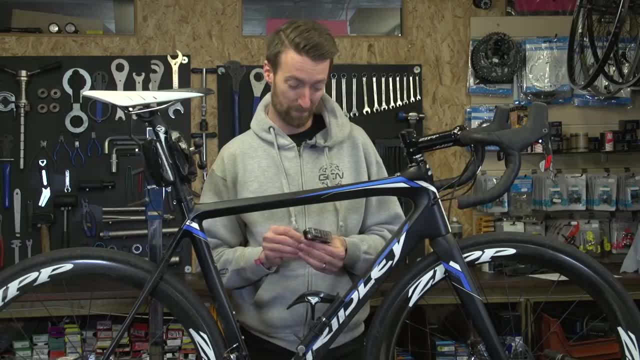 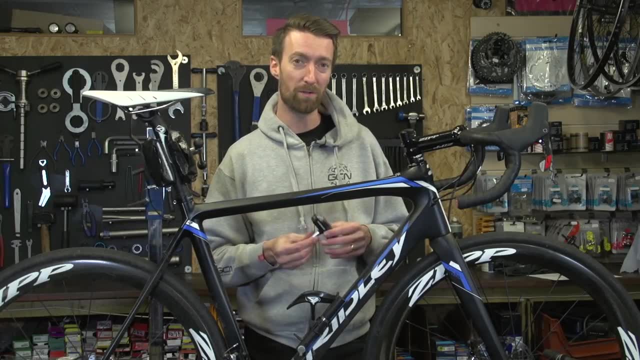 Now the next thing that you can do to prolong the lifespan of your bike is to use a torque wrench. You might be wondering how, but I'm about to explain. Now, these are becoming increasingly important when it comes to tightening bolts on lightweight components, and particularly carbon components. 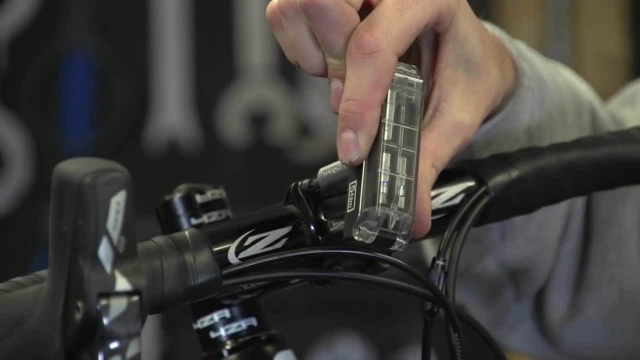 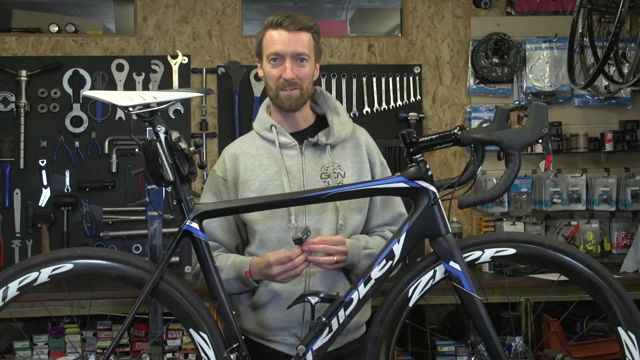 because over-tightening these parts can lead to extra stress, which ultimately, in a worst case scenario, can lead to complete component failure, which is, of course, the last thing that you want to happen when you're out riding your bike. Now, the good news is that you can pick up. 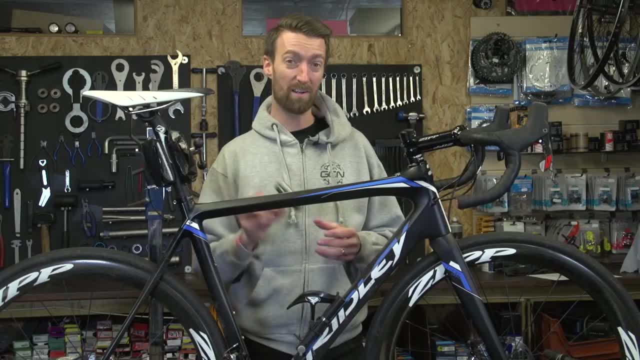 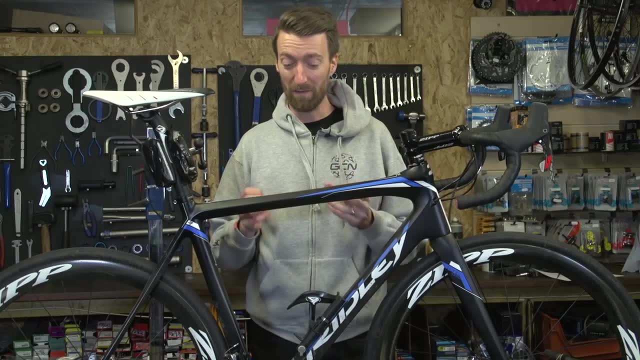 something like this pretty cheaply on the market these days, and it should last you a very long time indeed. Another thing to watch out for with lightweight frames, and particularly carbon frames, is any kind of bike rack or bike stand which clamps around the tubes. 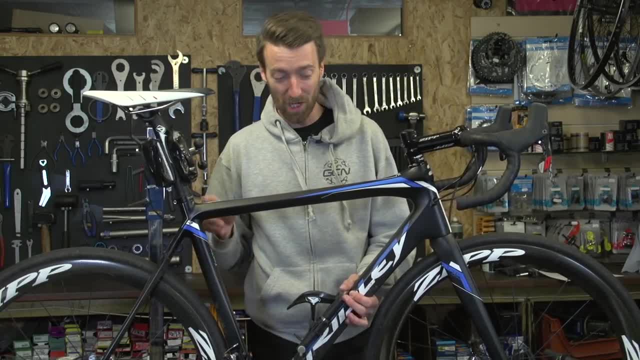 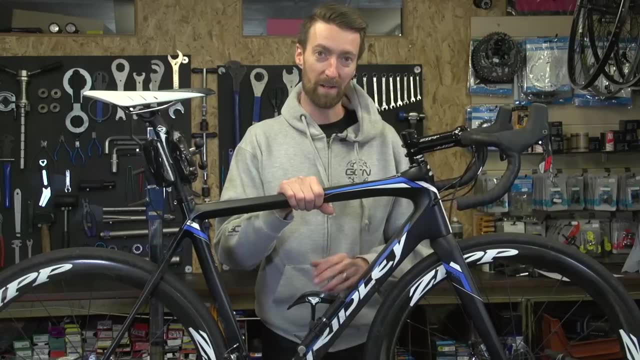 Top tube here, the down tube or the seat tube. Now, carbon frames are only designed to be strong in the direction that they need to be when you're out riding, but when something is clamping around it, that can lead to the tube being crushed or squashed. 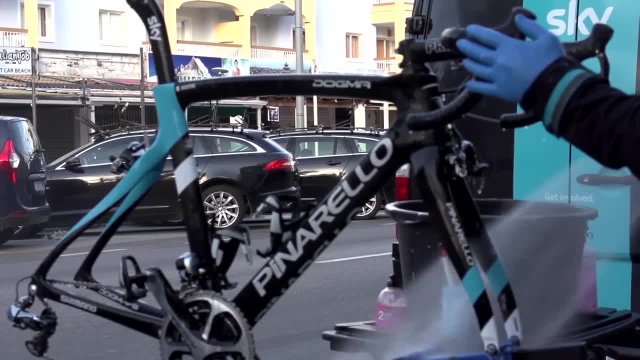 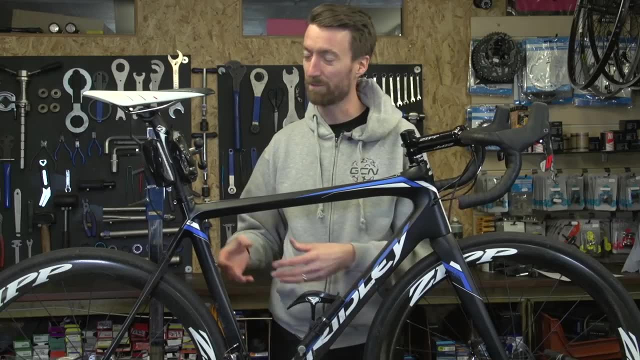 So what we would recommend is buying one of the stands like the pro mechanics use, whereby the forks go into the dropouts at the front and the stand then supports it underneath the bottom bracket. here, However, if you do have to use some kind of stand, 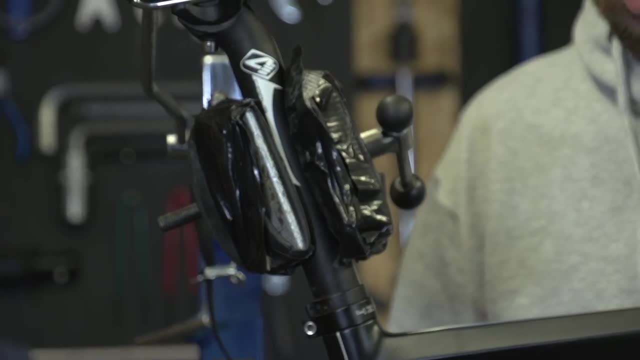 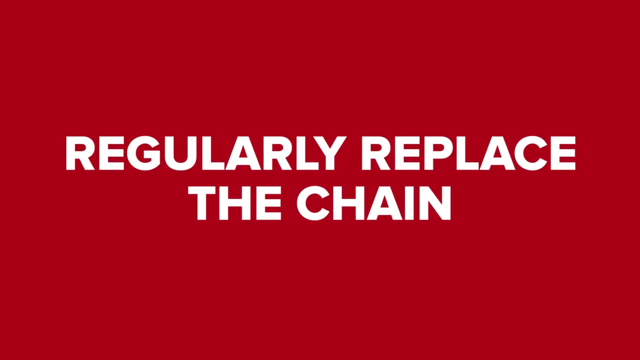 like this one, then we'd recommend clamping it at the saddle, not tightening it too much, and also adding some kind of cushioning so that you've got less chance of squashing the seat post. You also want to make sure that you change. 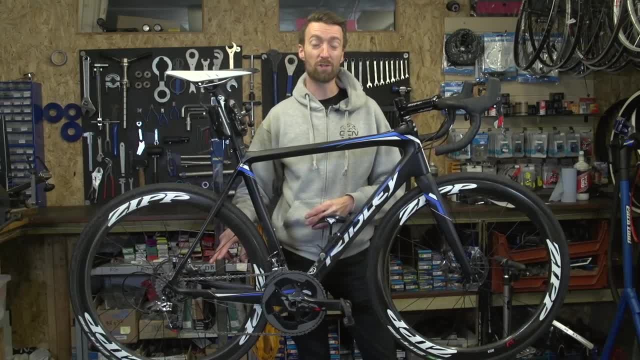 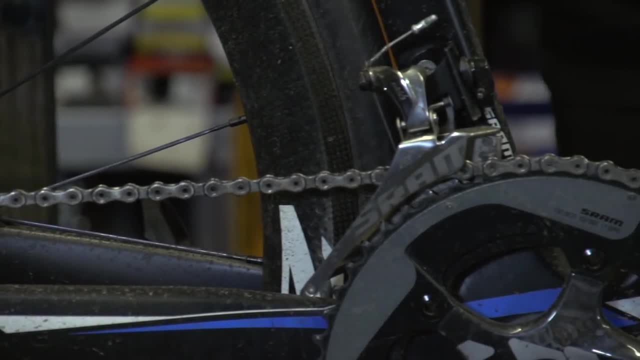 and renew your chain at regular intervals, And that's because over time, when you ride your bike, the chain will stretch slightly and wear, and in turn it will then wear the chain rings and also the cogs here at the rear cassette. What that means is that eventually, 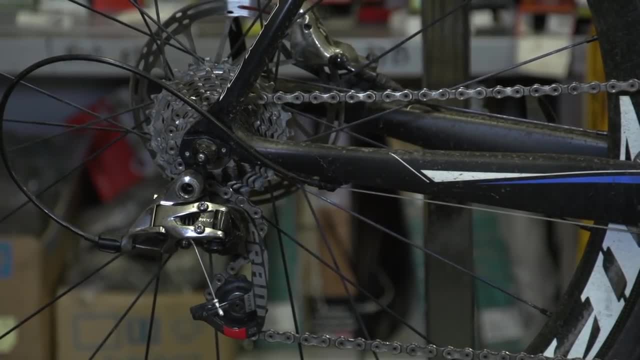 you're going to have to replace the whole lot, which can be far more expensive than replacing the chain every so often. Now, there are a few ways to measure the chain wear, and we've got a video that shows you how to do just that. 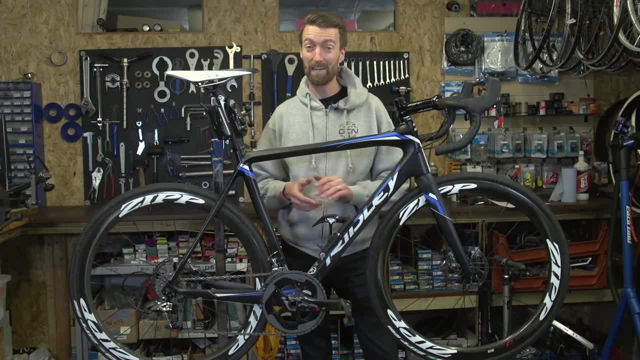 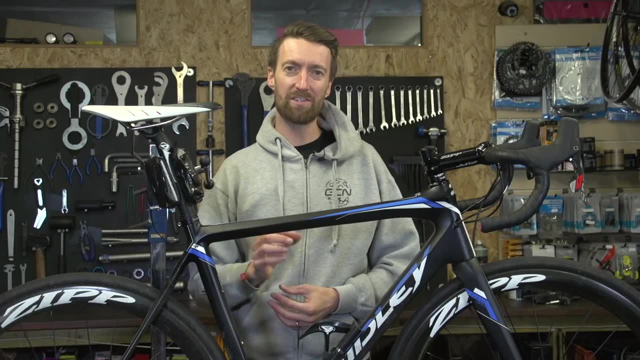 You can find a link to it in the description or in the description box below this video. Thanks for watching. I'll see you in the next one, Just below this video. Now, just as if you let your bike stay muddy and mucky after a ride, it won't do it any good. 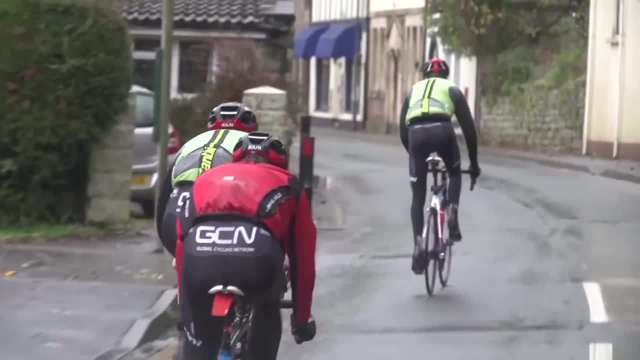 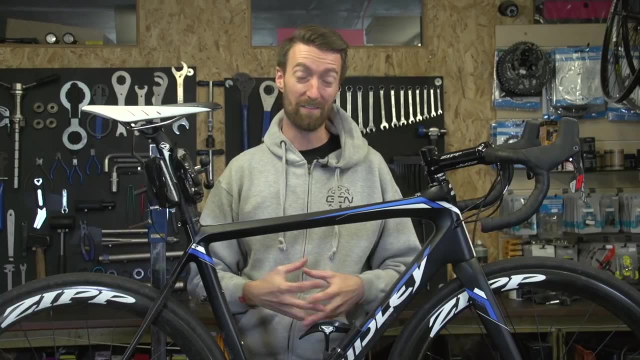 Also, riding down particularly mucky or gritty roads will wear all the components out far quicker. So when the weather's grim, if you've got an option, try riding on some slightly cleaner roads, And if there's no option, what you could do. 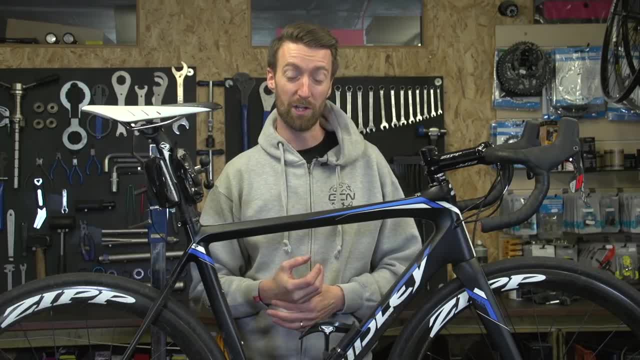 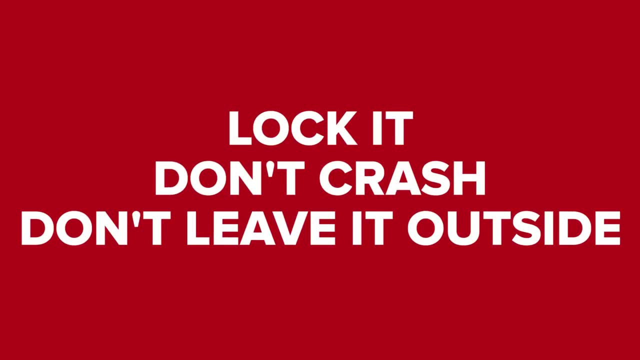 is invest in a much cheaper bike to use on days when the weather's not so good, which will mean that you keep your best bike in much better nick Right. we're going to leave you with three more suggestions, which almost go without saying. 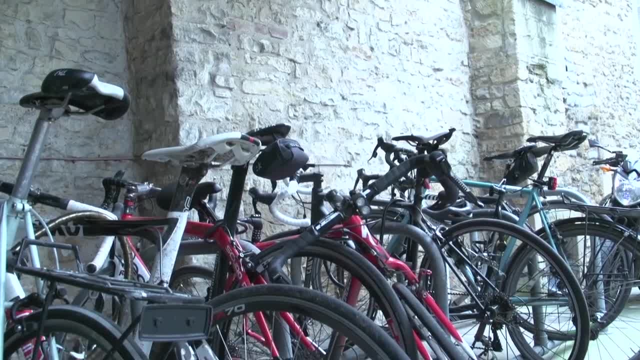 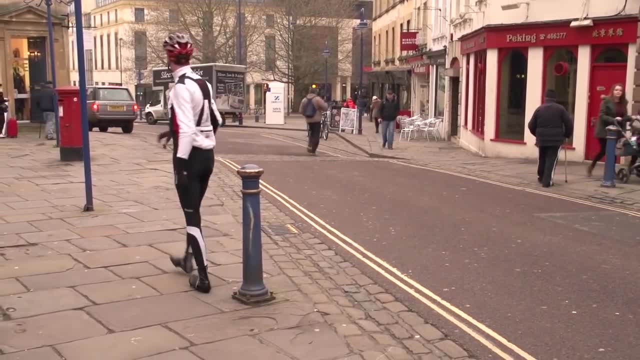 First up, whenever you leave your bike in a public place, make sure that you lock it up securely, And we're not saying that your bike won't last a long time if it's stolen. It's really not much good to you if it's in somebody else's hands. 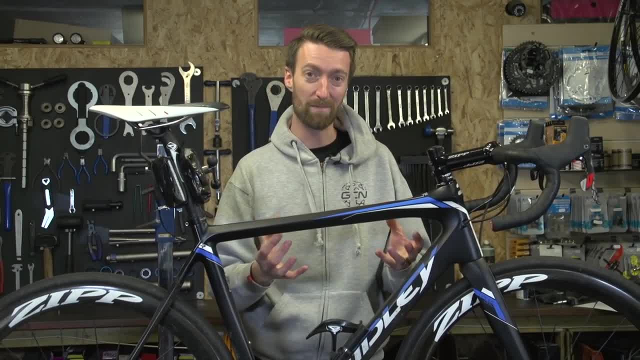 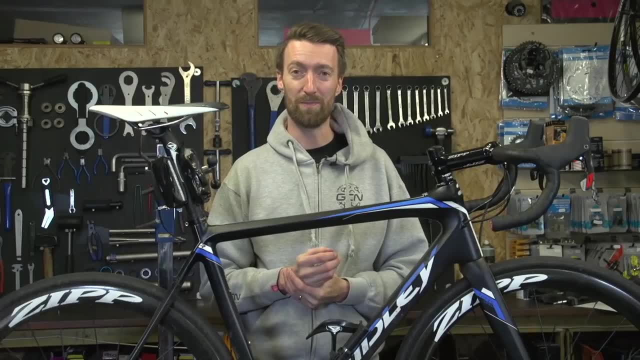 Secondly, try to avoid crashing. Lightweight carbon frames such as this one really aren't designed to take huge knocks, So a crash could hurt your wallet just as much as it hurts your body. And finally, try to keep your bike stored indoors, or at least under cover. 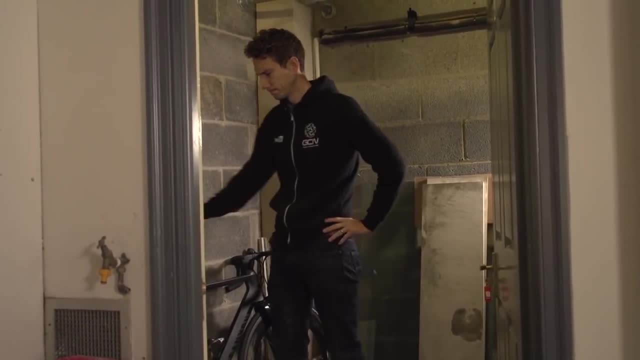 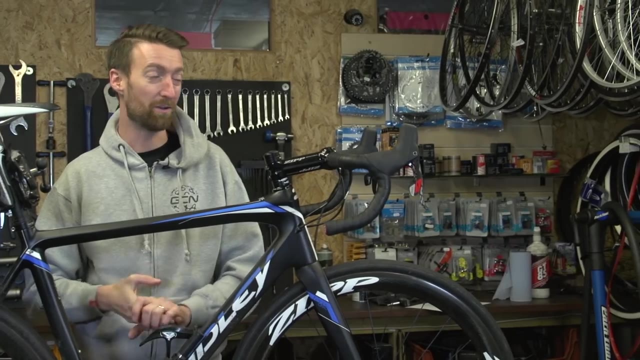 Leaving it outside and exposed to the elements is only going to speed up the aging process of the bike as rust starts to set in. Now, if you would like to see our video which shows you how to do a really good 30 minute thorough bike wash, 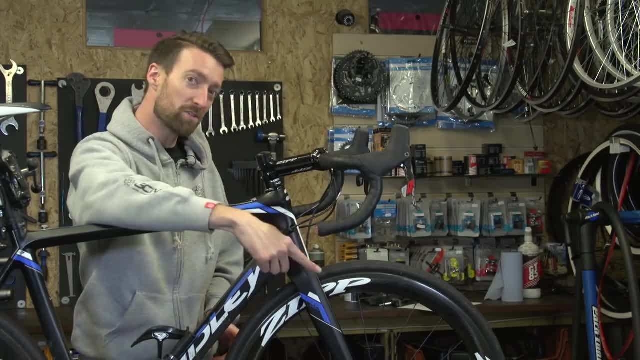 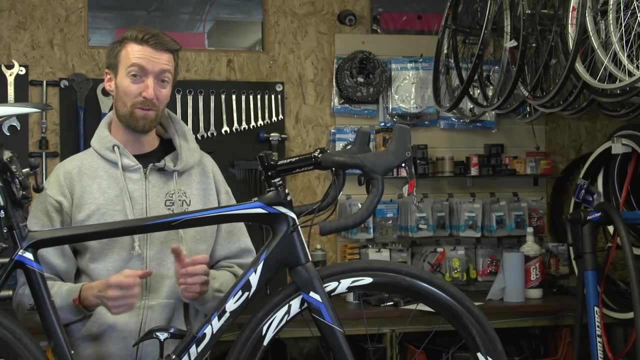 you can find that just in the top corner there. Meanwhile, just in the bottom corner is our advice on how to use a torque wrench. Or you might want to subscribe to the channel. It's free. There's going to be loads more videos, just like this.